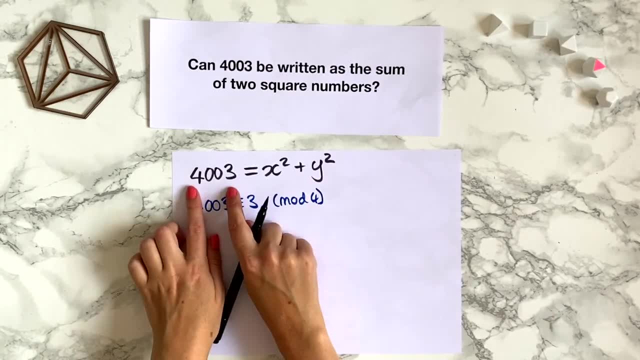 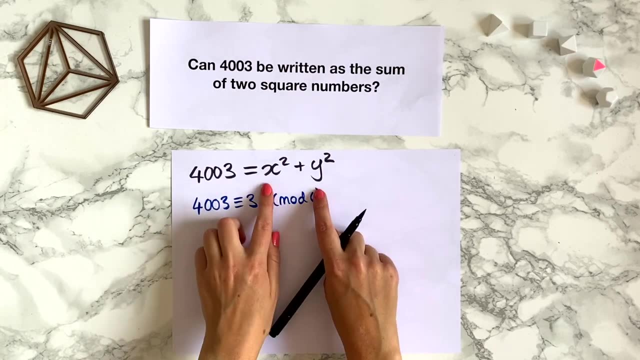 numbers x and y, such that x squared plus y squared equals 4003.. Because x squared plus y squared equals 4003. this means that 4003 is congruent to 3 modulo 4.. So 4003 is congruent to 3 modulo 4.. But x squared plus y squared must also be congruent to 3 modulo 4.. 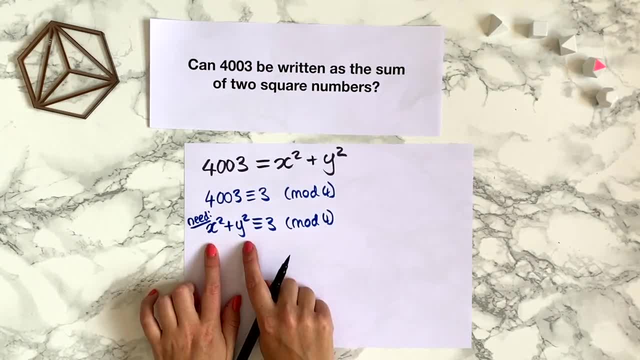 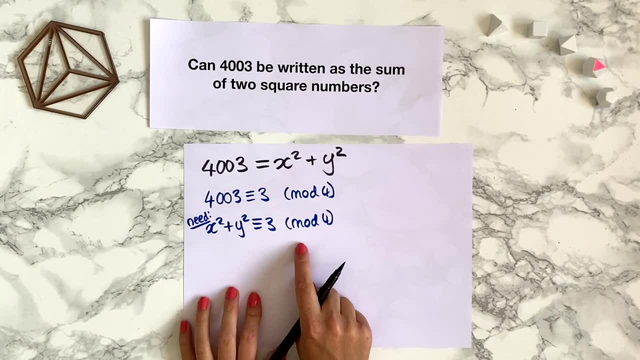 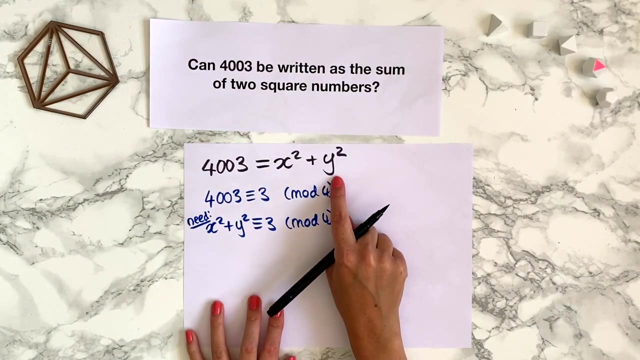 Now this is interesting. Let's check that that is actually possible. Is it possible to have two square numbers added together and that sum is congruent to 3 modulo 4?? Because if that's not possible, then we can't write 4003 as the sum of two square numbers Now in modulo 4,. 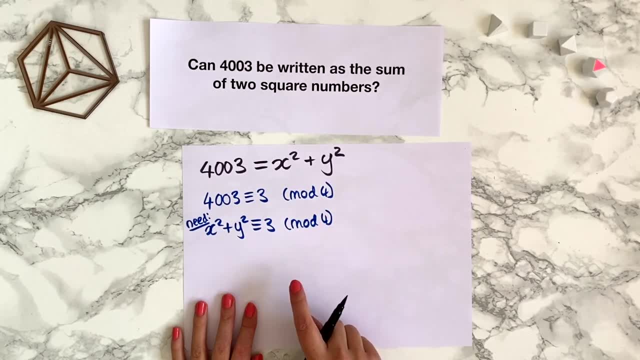 numbers can be congruent to either 0,, 1,, 2 or 3.. They've got four options of where they can be on the clock. So modulo 4, x and y are each 1 or 0,, 1,, 2 or 3.. Now let's see what that means for. 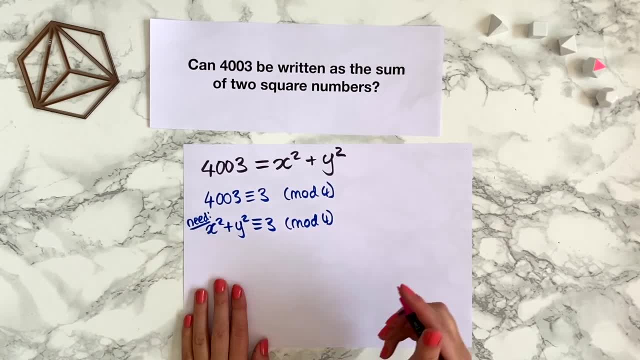 what x squared and y squared are. So in modulo 4, say x or y is 0. So let's just focus on x values. So let's say x. we're going to make a table here. We're going to have 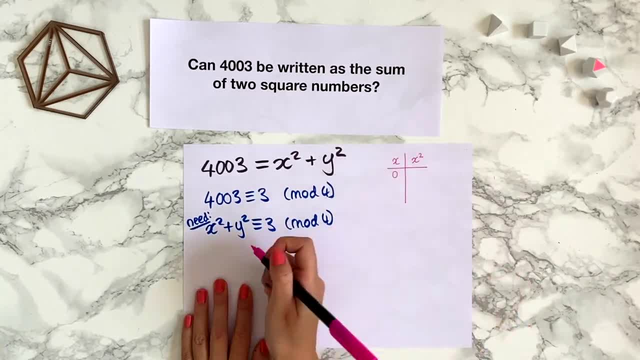 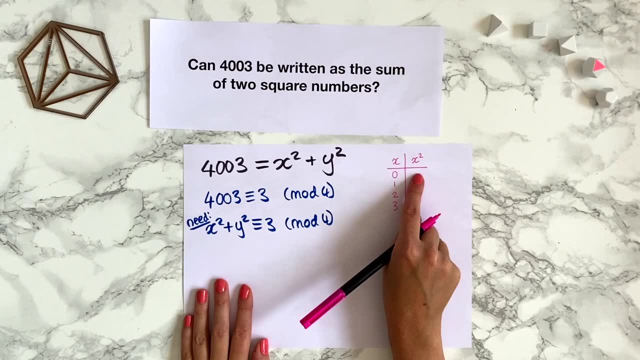 x in this column and x squared in this column, So x can be either 0,, 1,, 2 or 3 in modulo 4.. So if x is 0, x squared modulo 4 is still 0.. If x is 1, x squared modulo 4 is also 1.. 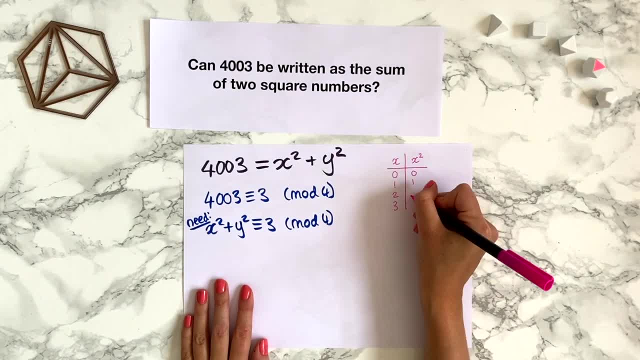 If x is 2, x squared is 4, but that's congruent to 0 mod 4.. So this is a modulo 4 table. Everything we do is going to be filhoïd and we're going to reduce modulo 4.. If x is 3, then x squared is 9. 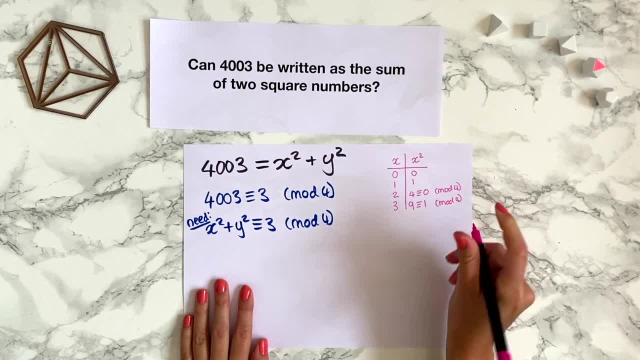 and that's congruent to 1 modulo 4.. 9 leaves remainder one when you divide it by four. So that means in modulo 4, this x squared can either be 0 or 1.. It can take any other values, modulo 4.. 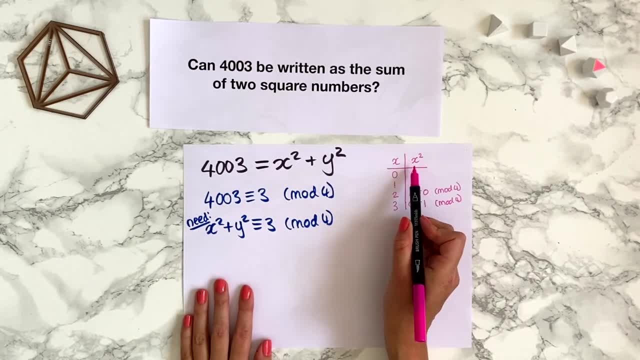 But this is exactly the same as if we did it for y. If you put y here and y squared here, y can also only take the values for y, 0,, 1,, 2, and 3 in modulo 4, so y squared can also only take values 0 or 1 modulo 4.. 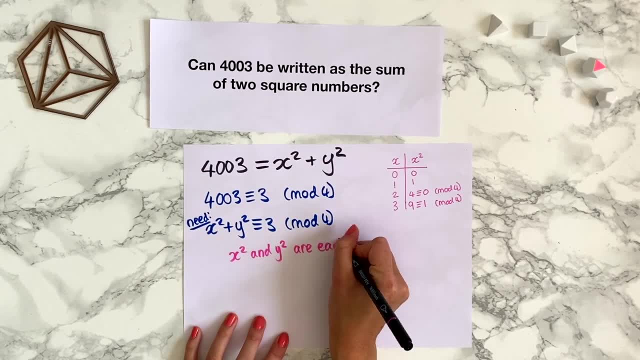 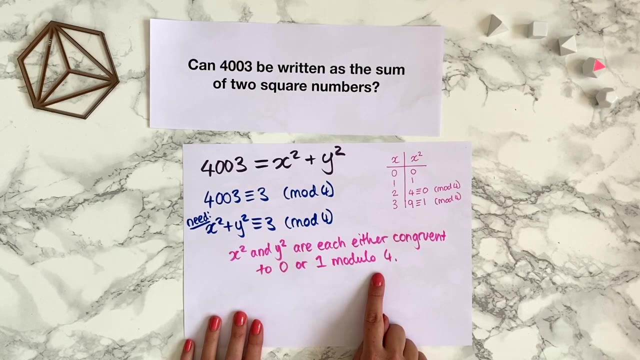 So we've shown that x squared and y squared are each either congruent to 0 or 1 modulo 4, regardless of what number they represent. those are the only possible values for a square number modulo 4.. But then x squared plus y squared can't be congruent to 3 modulo 4, because no combination. 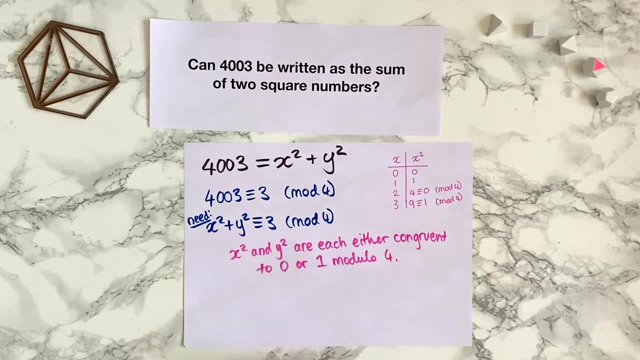 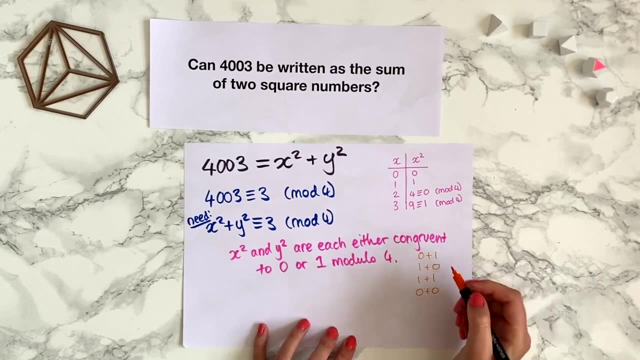 of two of 0 and 1s add to make 3.. For instance, 0 plus 1, or 1 plus 0, or 1 plus 1, or 0 plus 0, neither of these make 3.. So it's impossible for x squared plus y squared to be congruent to 3. 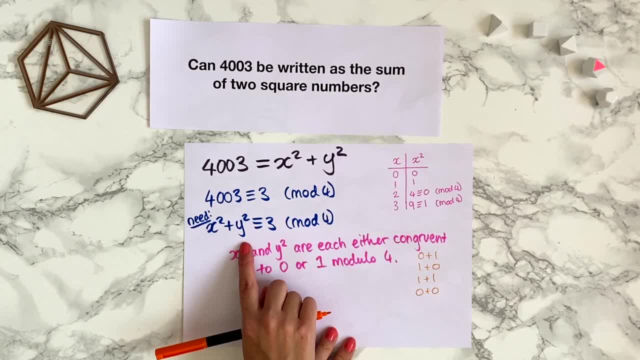 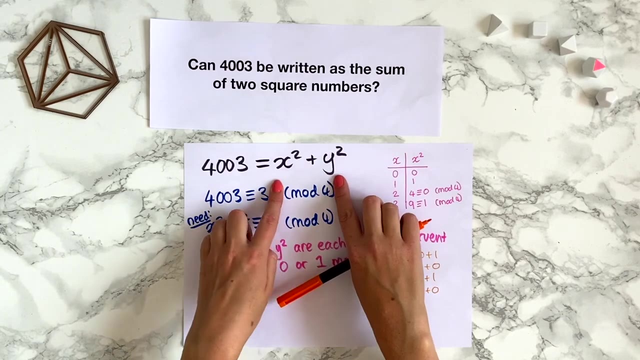 modulo 4 for any value of x and y. So this proves that 4003 cannot be written as the sum of two square numbers. So what we've done here is a proof by contradiction. We've sort of said: let's suppose that 4003 can be written as the sum of two square numbers. 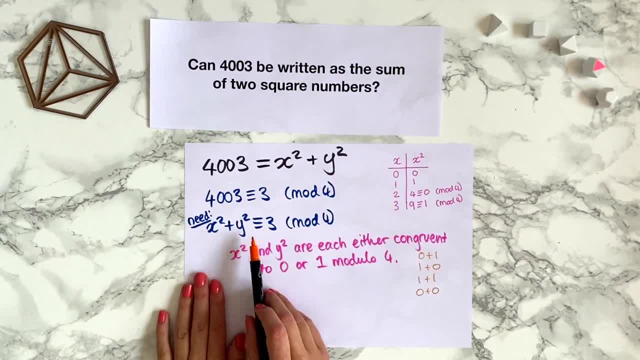 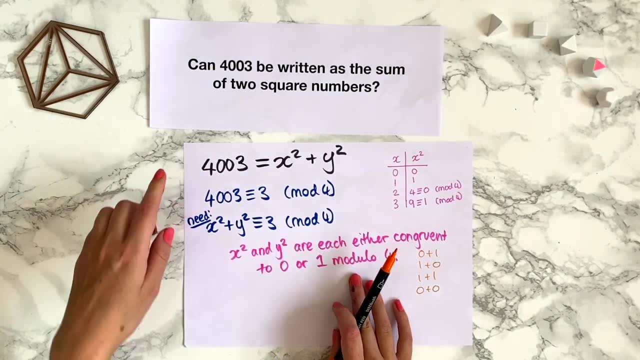 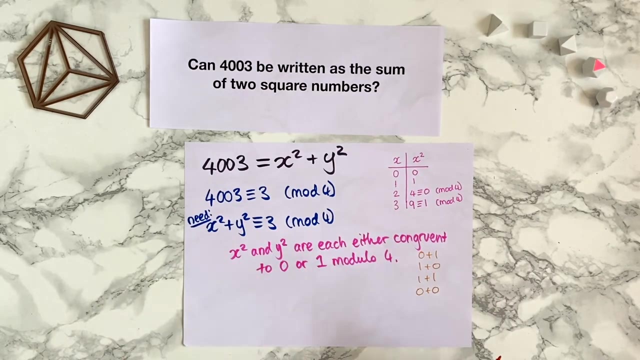 in which case we would have to have that x squared plus y squared is congruent to 3 modulo 4, simply because 4003 is and these two things are equal. But then if we look at the values that square numbers can take modulo 4, it turns out that square numbers can either be 0 or 1,. 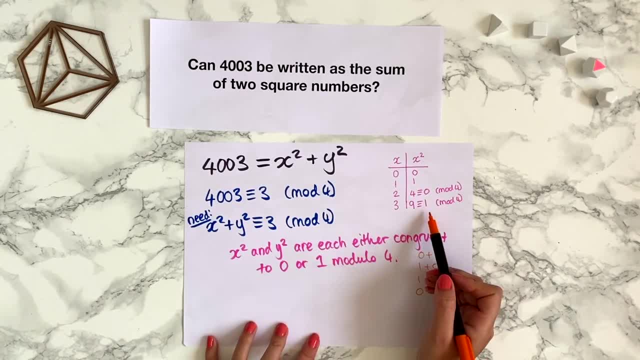 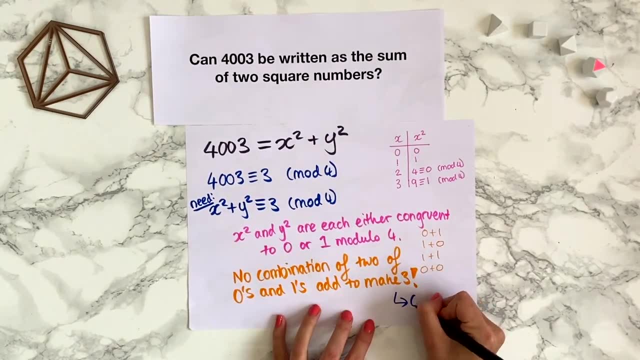 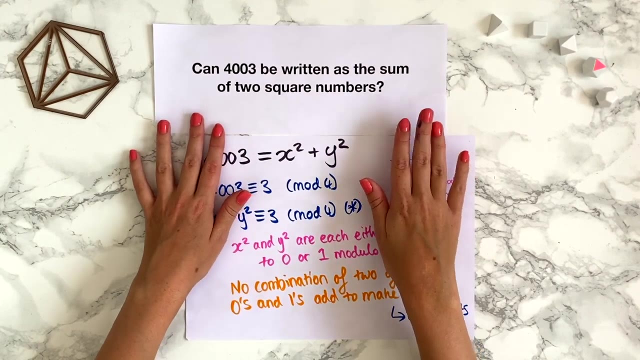 they can't be 2 or 3, just by looking at this table: No combination of two of 0 and 1s add together to make 3.. So we've reached a contradiction which shows it's therefore impossible to write 4003 as the sum of two square numbers. 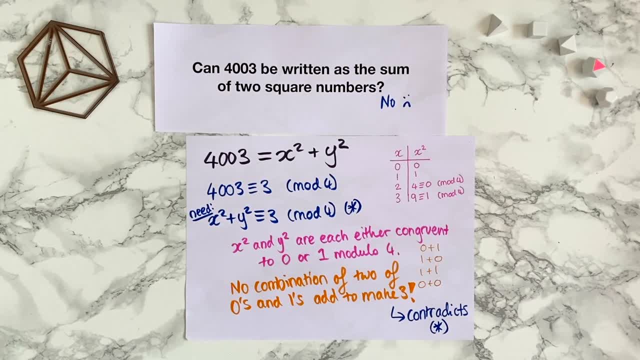 So we can use modular arithmetic to prove things as well as do calculations. You might be wondering how I knew modulo 4 would work. Well, if modulo 4 hadn't worked, we could have tried other modulos and seen if we could get a contradiction in a similar way.